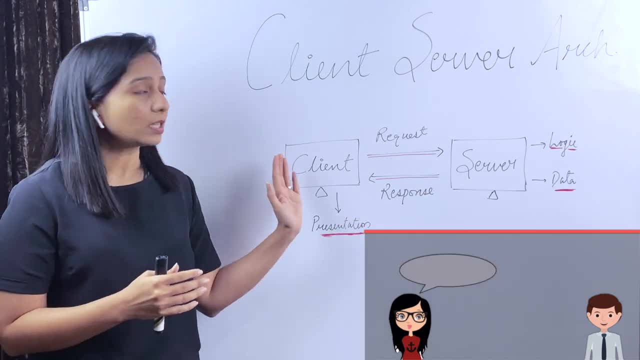 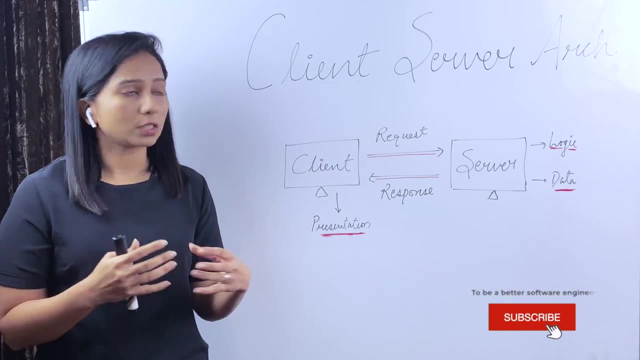 so, and so is the price of the property that you are interested in. This is basic client-server architecture, where server is responding to data. Now there can be scenarios or there are cases where some logical manipulation has to be done over the data. For example, there is a website. 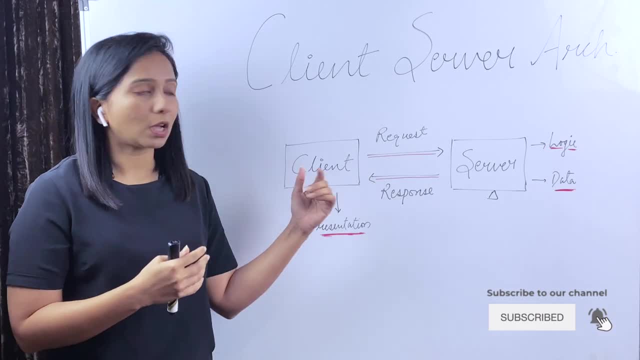 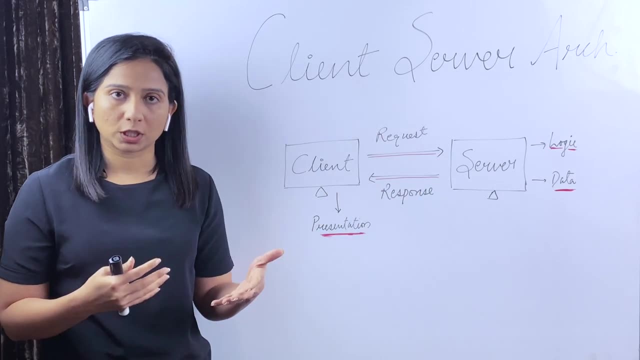 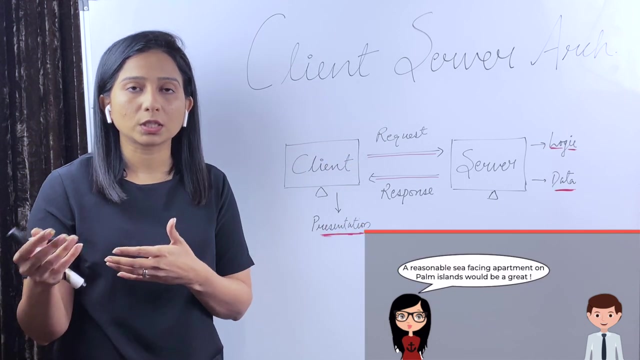 where I enter the yearly income and in response, after doing some logical manipulation and calculations on my income, the server responds with how much tax I have to pay for that year. For example, I ask the broker that this is my budget and I want to live in this area. Can you tell me what? which are the houses that I can afford? 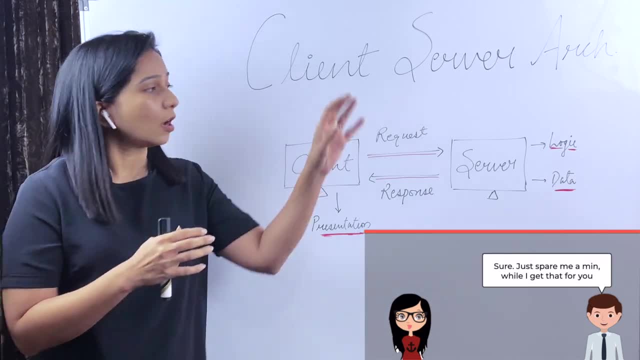 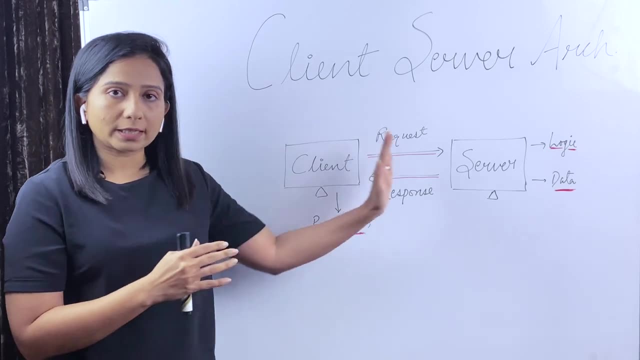 given in this budget. And then the broker takes my requirement, finds out all the houses and gives me a filtered list of the apartments. So now there is a logical manipulation done there. In basic client-server architecture, either it can be simple responding of data or there can be logical. 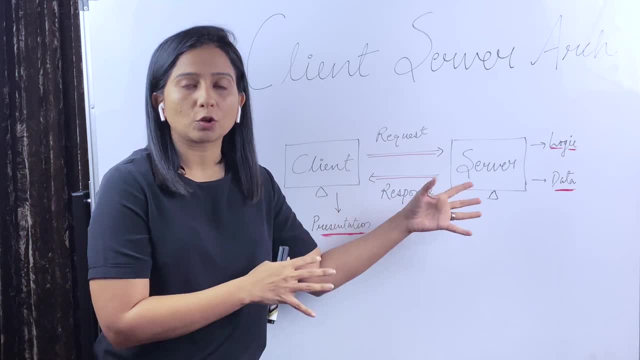 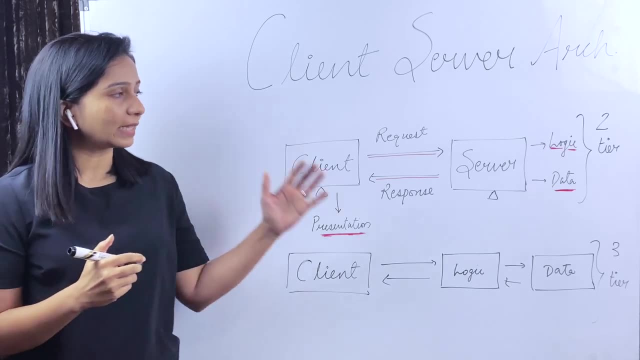 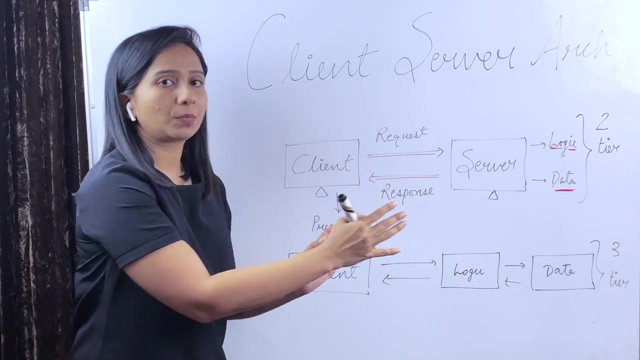 manipulation also be there, and the logic and the data both sit on the server. So that was a basic two-tier architecture. Important thing to note here is it is not always necessary that the logic sits in server. It might so happen that the logic, the logical manipulation or the processing 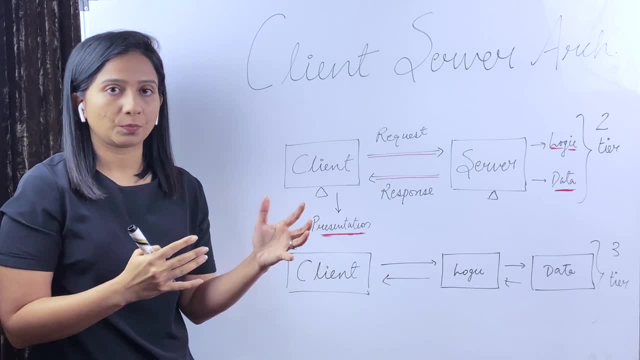 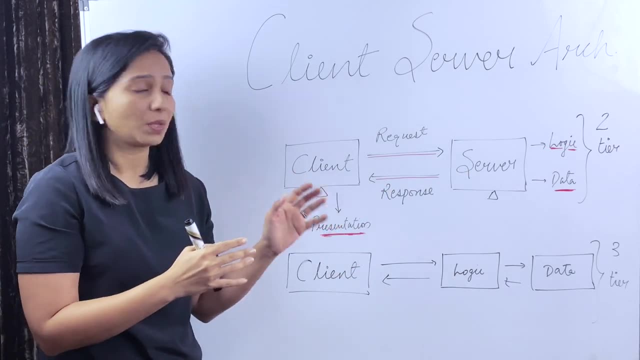 sits at the client side, That is called a thick client, And when the logic and the processing sits on the server side, that is called a thin client, because client doesn't have many responsibilities. Some example of thin clients are like streaming platform, Netflix or Hotstar. 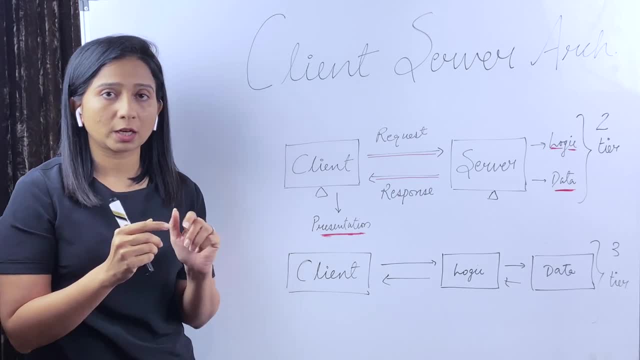 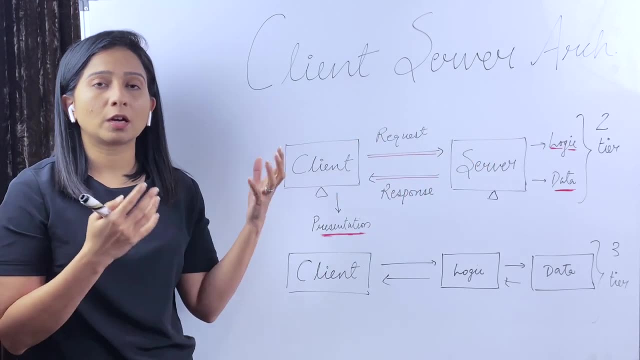 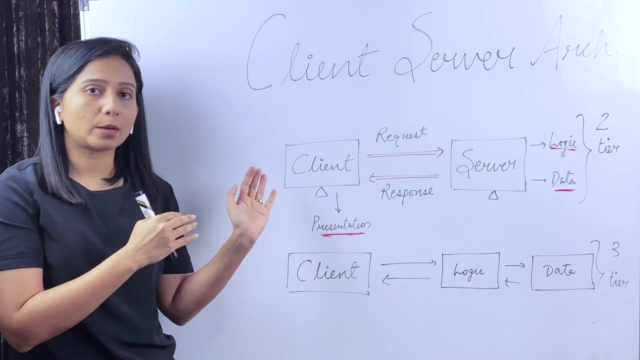 etc. In those cases, even though there is a presentation there, but the majority of processing happens on the back end or on the server side. So those are examples of thin client, Thick clients. on the other hand, applications like Microsoft Outlook or video editing software, where the majority of processing happens on the client side, are examples. 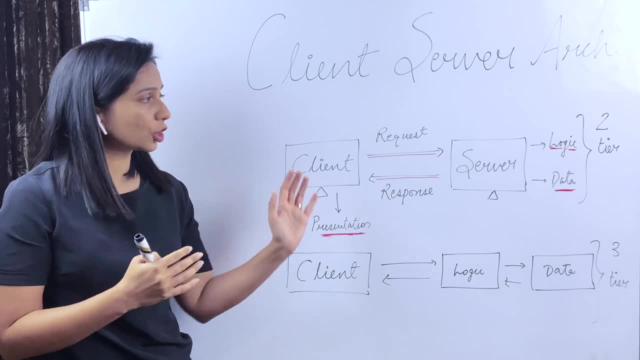 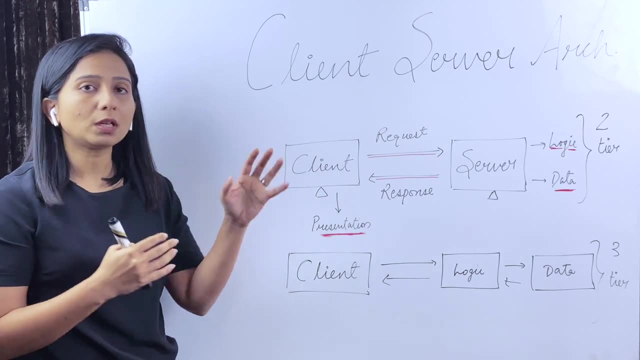 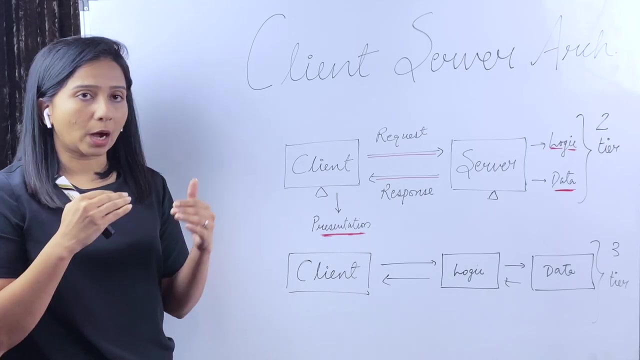 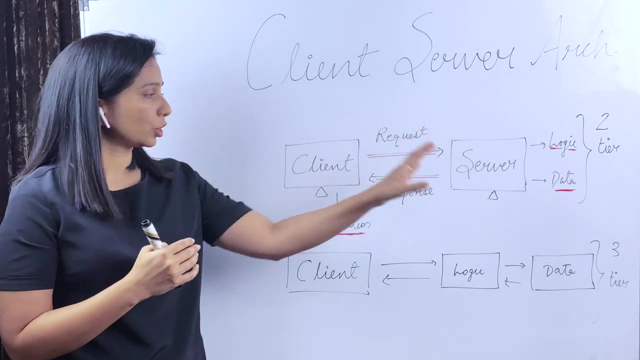 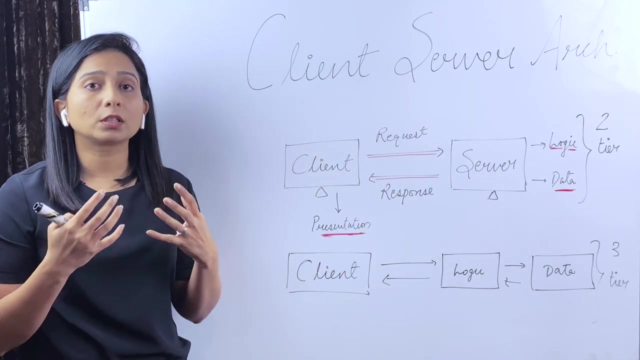 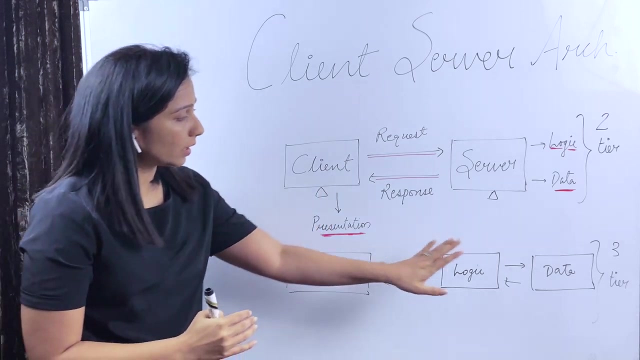 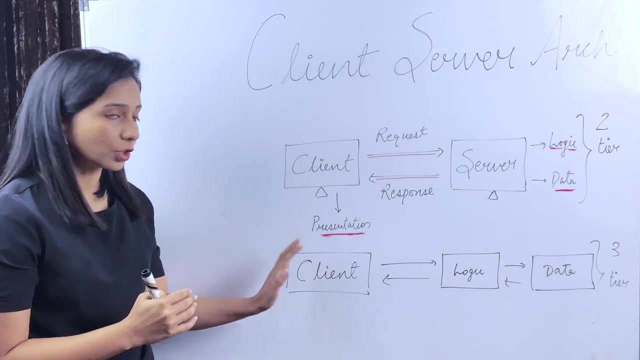 of thick client. So now, to summarize, there are three things: presentation, logic and data. Depending on where the logic and data sits or where the processing is happening, there can be thick client and thin clients. Up until now, we are talking only about two tiers, where there is client and there is server. The logic and data either sits on the server side or the logic sits on the client side. In the cases where the processing is huge and it has to be done on server side, or in the cases where the data is heavy, there is a lot of amount of data that has to be stored and processed- These two layers are broken. And then there is a logic layer, which is usually the application, And then there is a data layer, which is usually the database. In that case, this two tier architecture is broken. And then there is a logic layer, which is usually the application, And then there is a data layer, which is usually the database. In that case, this two tier architecture is broken. And then there is a logic layer, which is usually the application, And then there is a data layer, which is usually the database. In that case, this two tier architecture is broken, And then there is a logic layer, which is usually the application, And then 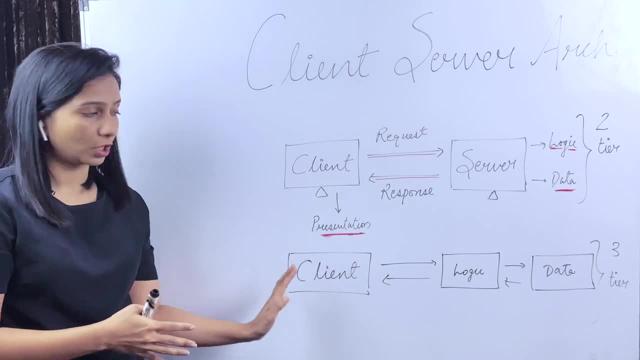 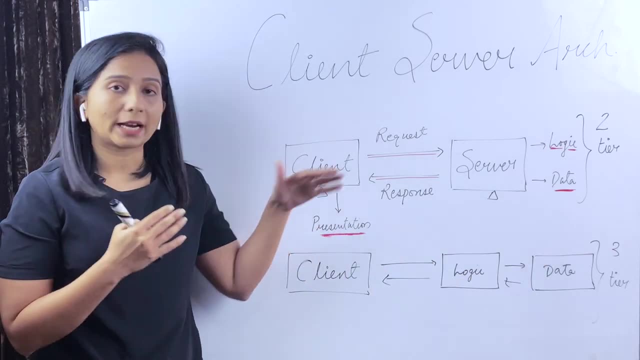 becomes a three-tier architecture. so now there is client, the presentation, there is logic or the application, and there is data layer, which is the database. so this is how different clients of architecture is designed in different tiers. in some cases even three tier is not enough. and then 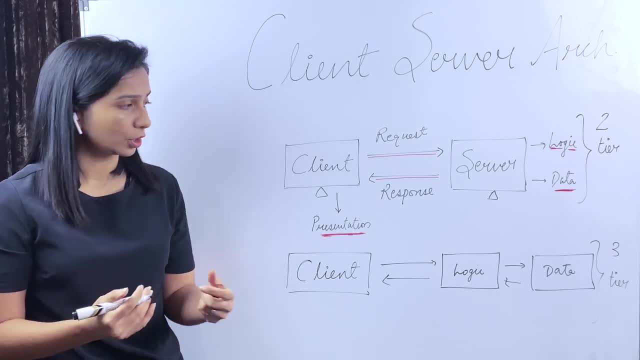 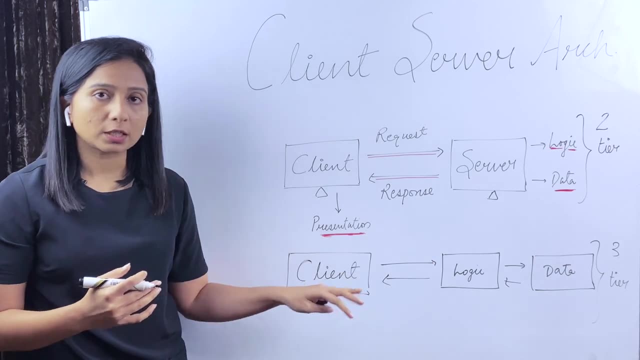 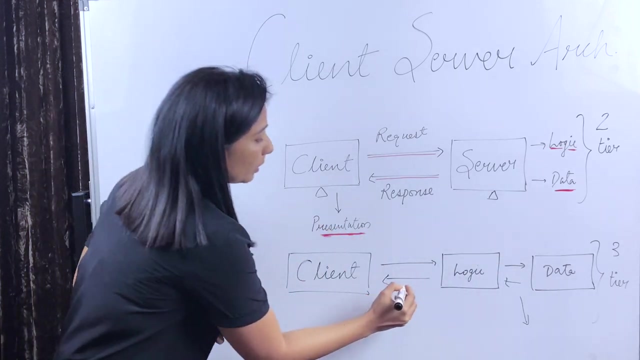 when you go on to design large and complex applications where even the processing and the requirement cannot be fulfilled in an efficient manner using just these two layers, then there are multiple layers in between. for example, a caching layer is introduced between the logic and the data layer, or there can be load balancers and proxies between the client and the 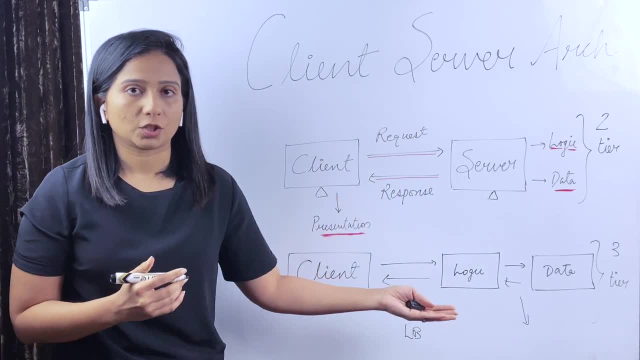 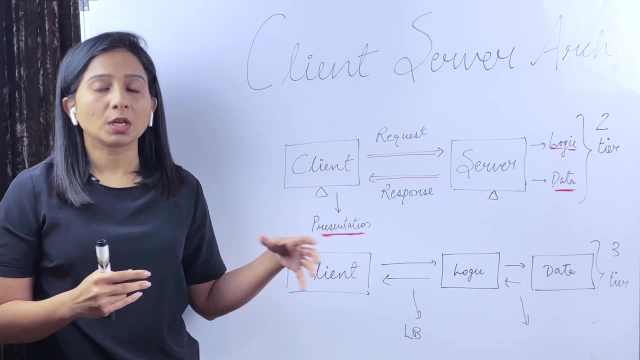 logic layer. those are the examples of n-tier architecture. now that we understand the basic of client-server architectures- different tiers and what are the different layers that are needed- the question is, how do you decide if you have to select a thin client or a thick client, or you have 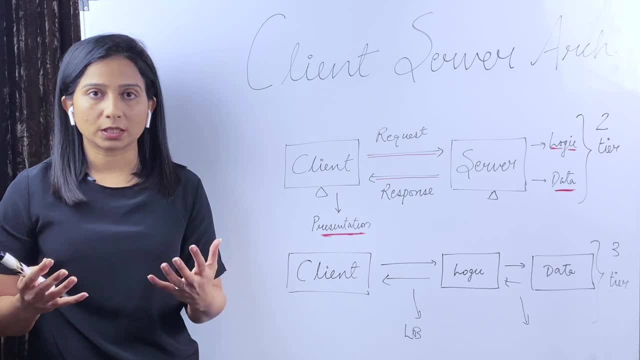 to go with a two-tier architecture or a three-tier architecture. it is very simple. if you have to go with a three-tier architecture, it is very simple. if you have to go with a, just have to serve images or text files and there is very less logical manipulation- you can go with. 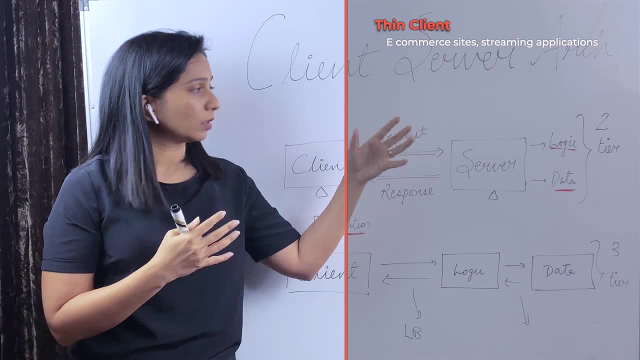 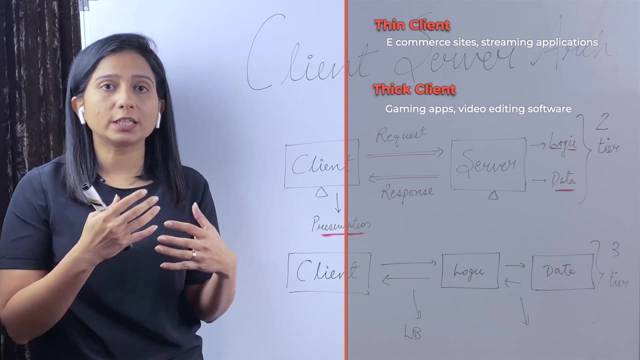 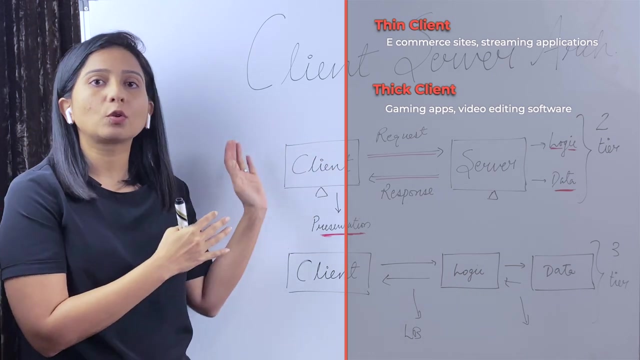 the basic lines of architecture where your server stores the information and serves the information. in case you are designing some rich graphical user interface or which which needs too much processing at the user end, like video games, etc. not online video games, desktop video games- in that case you can go with thick lines. in the cases where you want a rich graphical user interface,